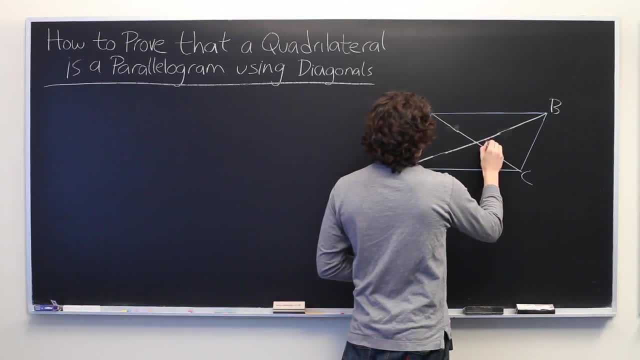 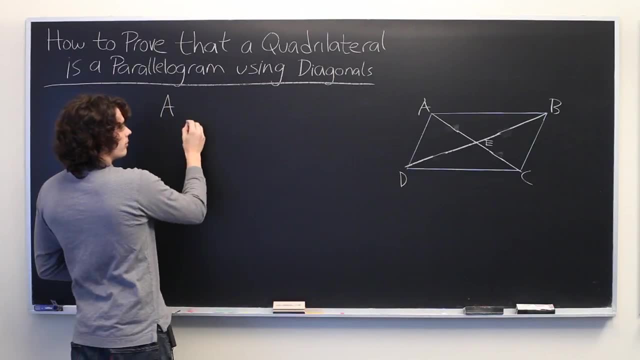 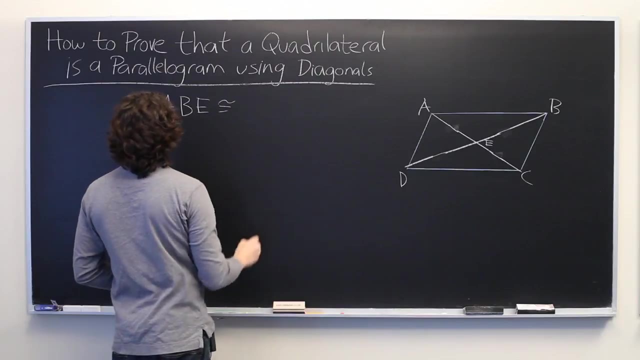 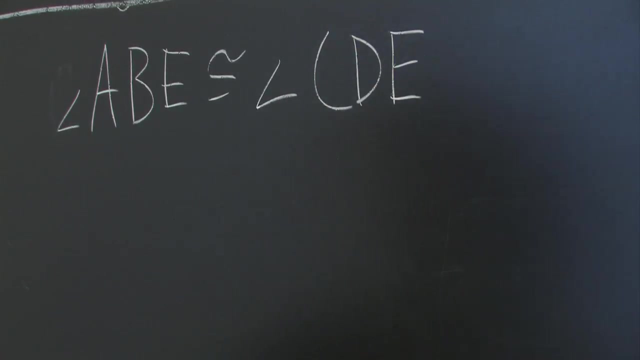 a, b, c, d, A, b, c, d And we'll call the centre e. Suppose that we are given that the angle a, b, e is congruent to the angle c, d, e And similarly we are given that the angle 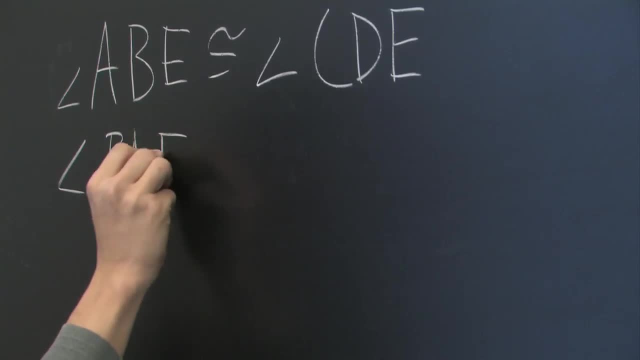 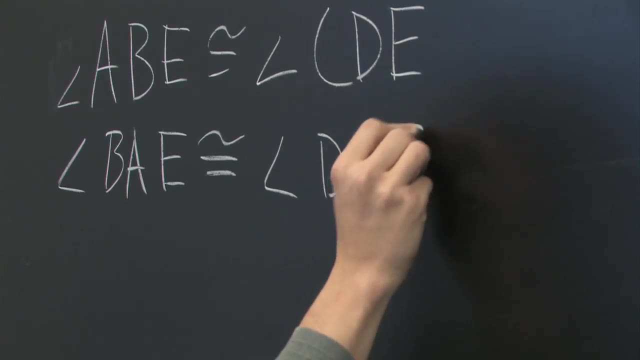 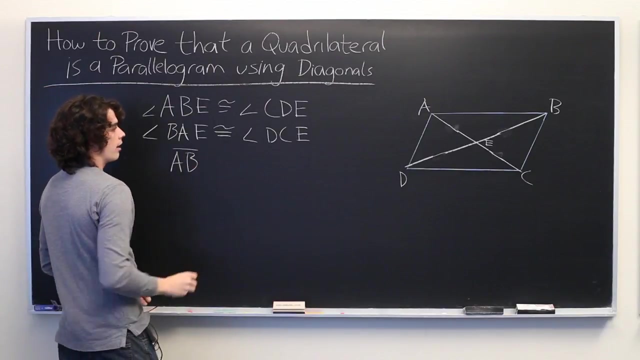 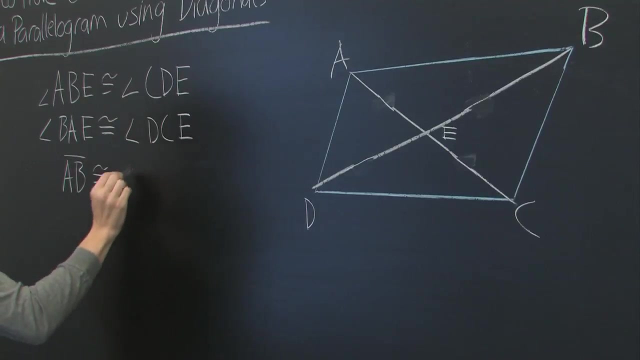 b, a, e is congruent to the angle d, c, e. And, lastly, we're told that the line segment a, b is congruent to the line segment c, d. Okay, let's go ahead and mark off the information. 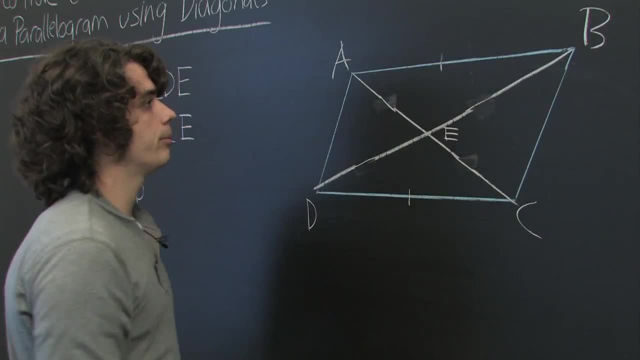 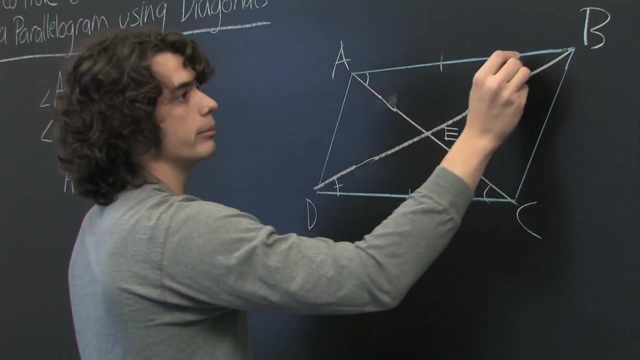 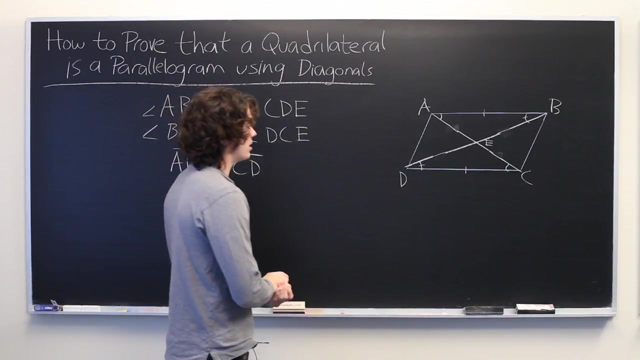 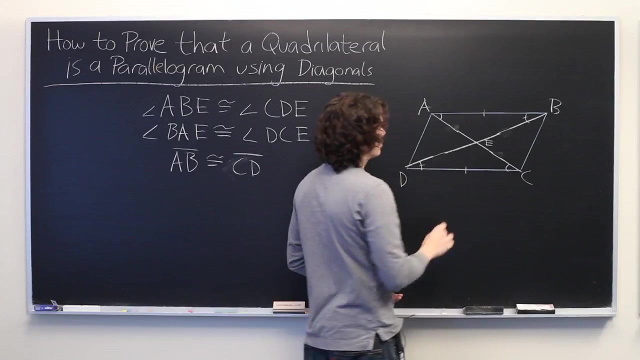 that we know. We know that these are congruent, we know that these are congruent and we know that these are congruent- Great. So, right off the bat, we can see that this triangle d, e, c is going to be congruent to this triangle b, a, e because of the a, s, a. 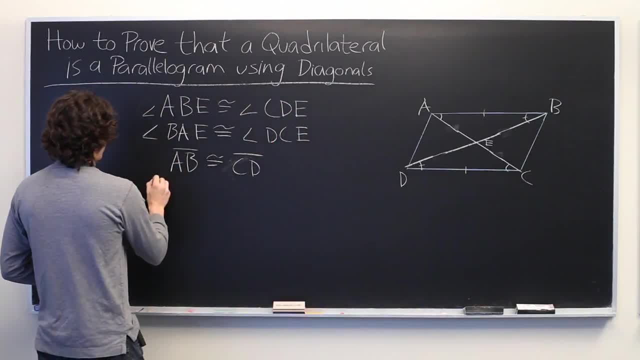 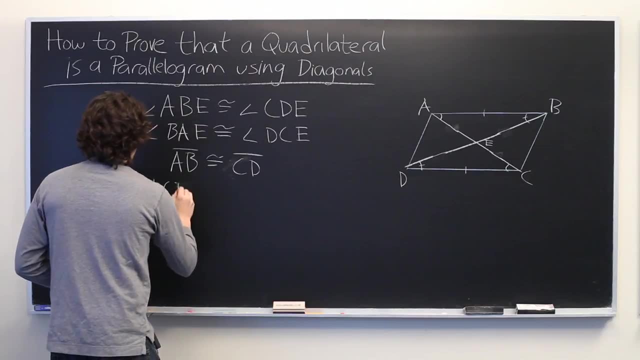 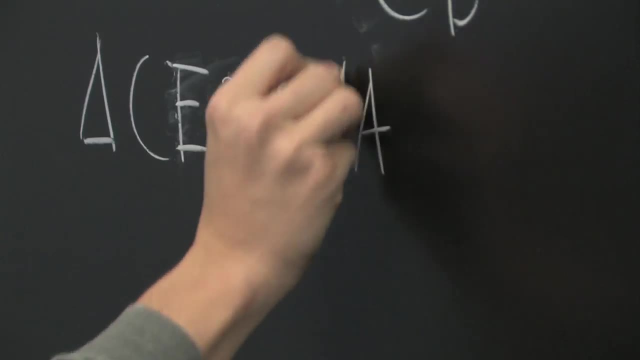 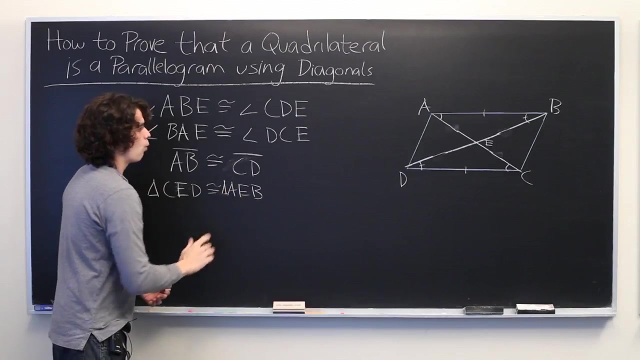 congruence postulate. So let's go ahead and write that out. write that down. We'll see in a second why that will be helpful for us. Triangle CED is congruent to triangle AEB. Okay, Well, from here we can quickly show that. this line: 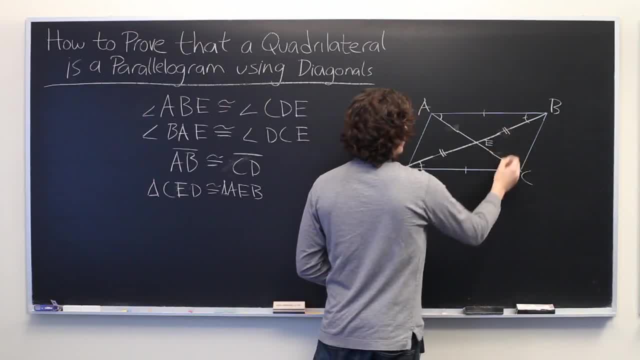 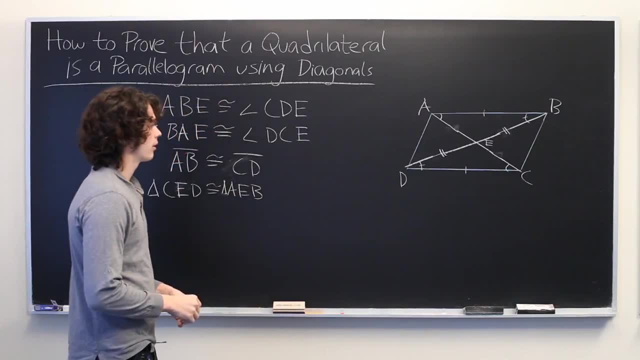 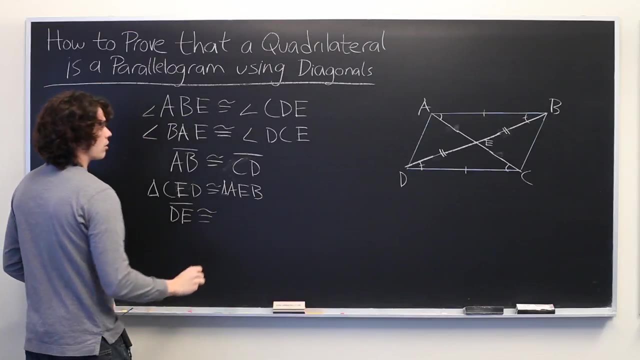 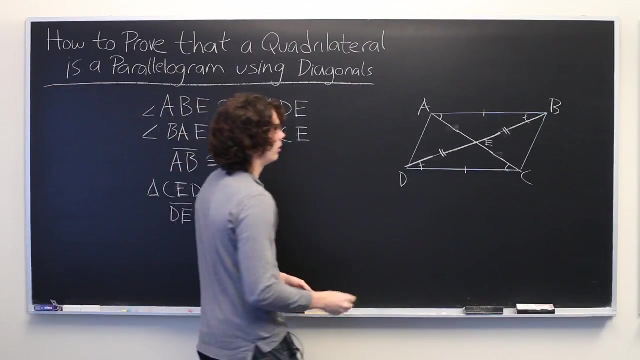 segment is going to be congruent to this line segment. by using CPCTC, Corresponding parts of congruent triangles are congruent. So we know that line segment DE is congruent to the line segment BE And similarly, we know that this line segment is going to be congruent.